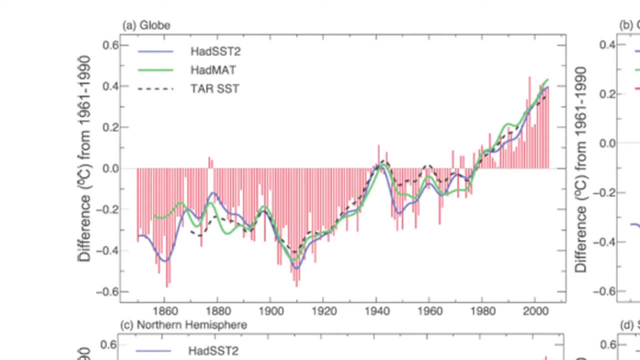 that this climate community has about this record of rises of changes in temperature from 1890 to about 1940,. there was a period of steady warming, not extremely fast falling temperatures in the intervening years- or perhaps steady temperatures- the interpretations vary- And then a renewed period of warming. 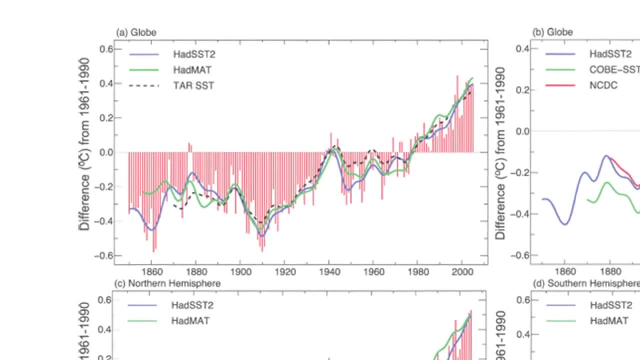 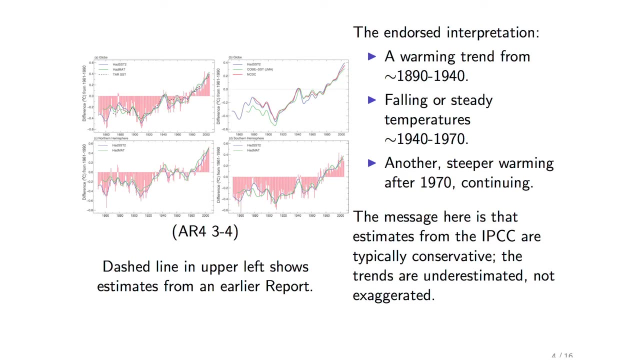 since 1970.. The reason I'm showing this figure is to remind you of that accepted interpretation, but also to note that in the fourth assessment report they looked back at what the third assessment report had shown And the evidence here suggests that the interpretation 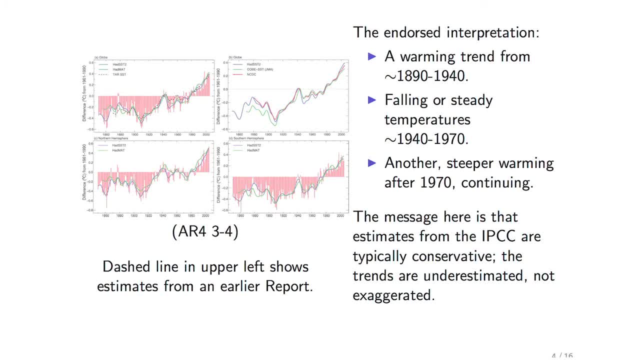 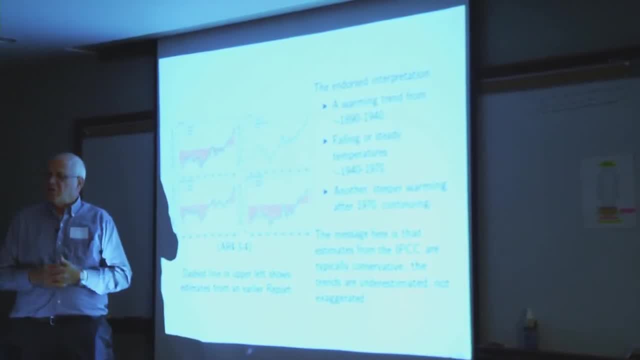 that the accepted wisdom by the climate community doesn't overestimate the effects. In fact, if anything, we tend to underestimate the effects. Scientists are, by their nature, conservative, in the sense that they try not to say things that they can't be sure of. 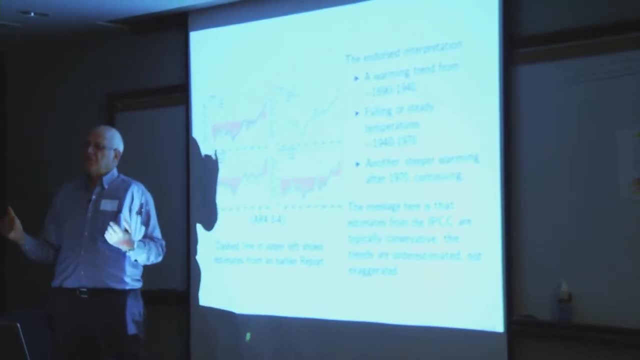 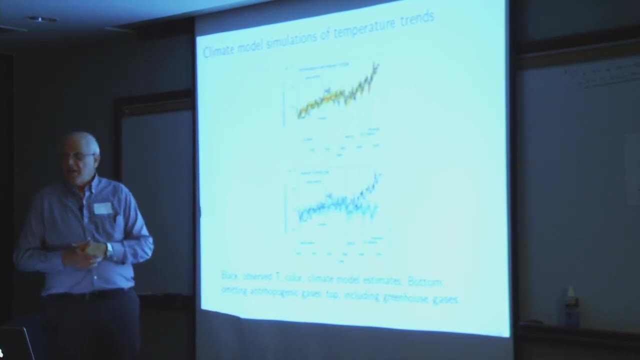 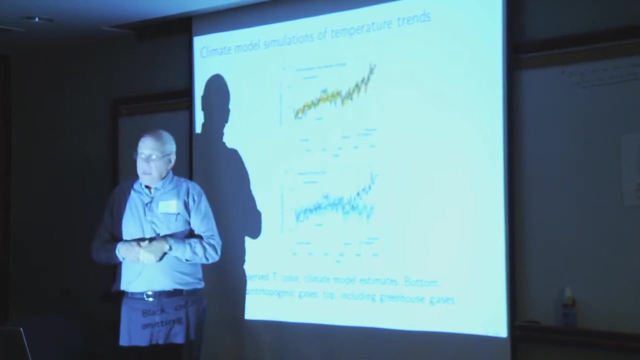 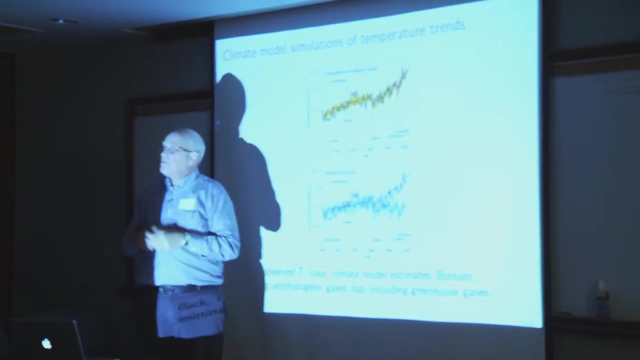 They hedge their statements to make them defensible in as strong a way as possible. This is a very different graph showing what appears to be a similar time series, an extended period of time, And the thin lines are observations, The thick lines are simulations. 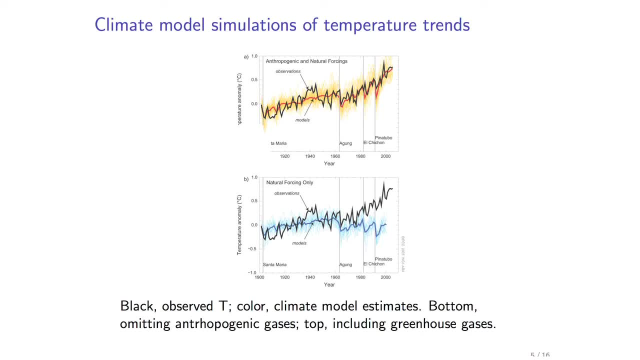 These are simulations by climate, So these are climate model estimates of the global average temperature in two very different sets of model runs. In this there were dozens of climate models that were used to simulate a whole century of climate, And the model runs were by design set up. 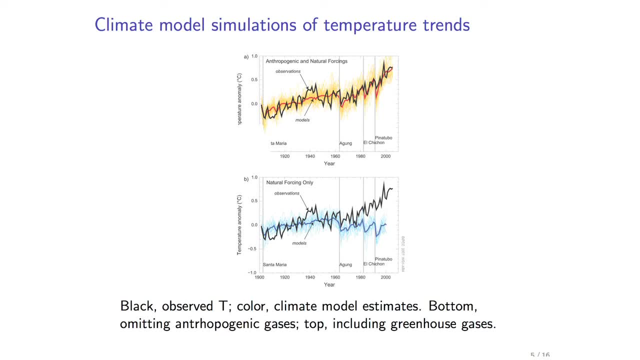 in two very different ways. One set of simulations Shown in the bottom is a counterfactual scenario, a scenario that doesn't match what happened in reality. In that set of simulations, the models turned off the emission of greenhouse gases by humans. 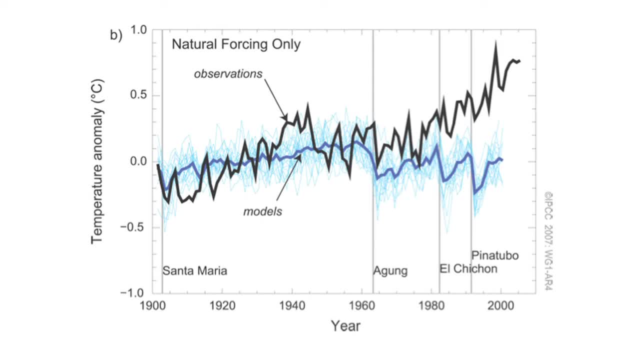 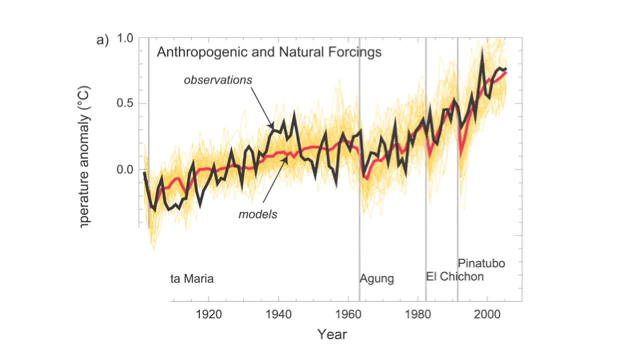 So we cut back as if everybody was an environmentalist starting in 1900.. Those simulations are shown in blue at the bottom. here In the upper panel we have a simulation in which all the effects of human-induced climate change were included in the model scenario. 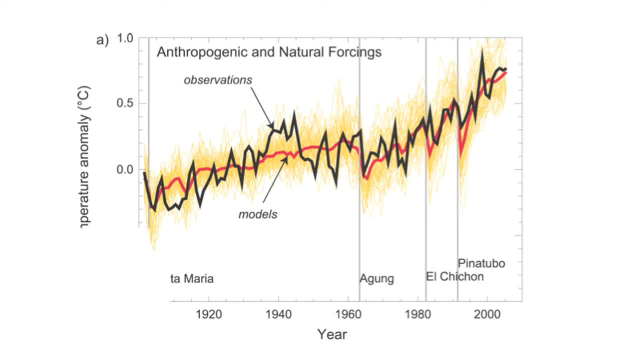 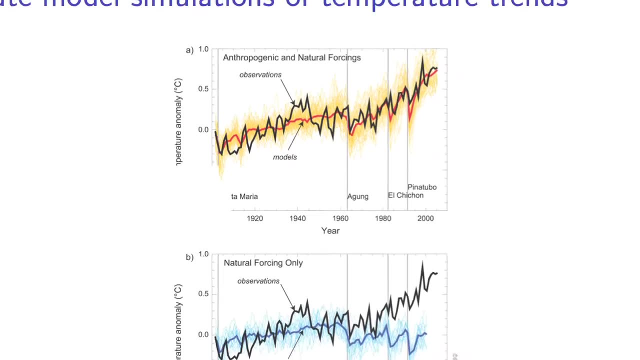 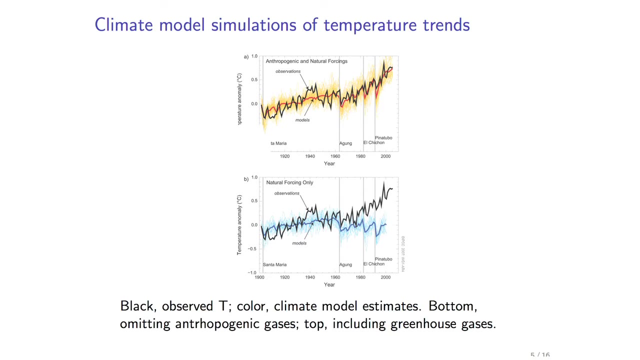 And the black observations. the line indicating the observations is the same in both cases. Look at the counterfactual simulations. When you don't include the anthropogenic greenhouse gases, the models indicate that this warming that we've observed, especially since 1970, wouldn't have occurred. 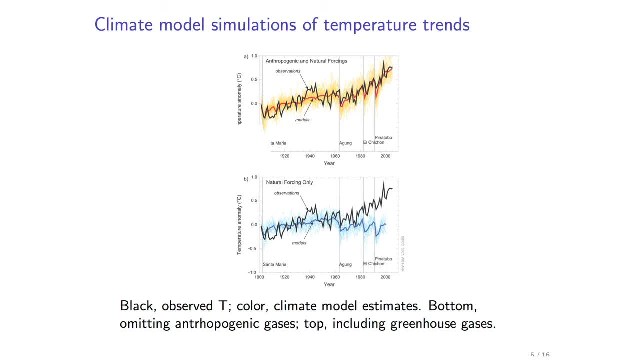 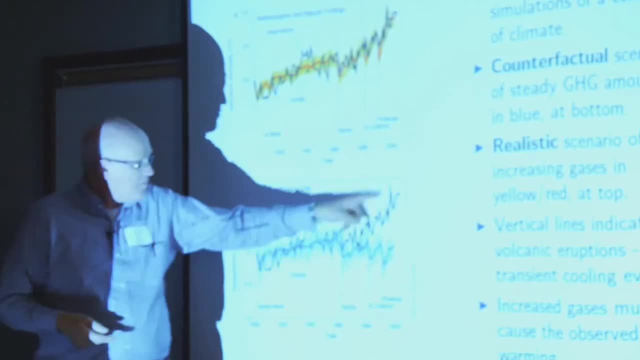 And so the models say we can't account for the warming unless we include the anthropogenic greenhouse gases. Another factor that's shown in this figure are the occurrence of major volcanic eruptions. This reminds us that nature is, of course, extremely variable. 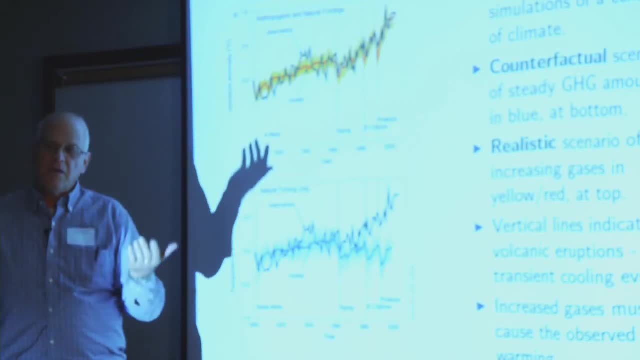 Volcanic eruptions cause global cooling by putting gases in the atmosphere which are oxidized to aerosols in the stratosphere, And so you see drops in temperature associated with that. When you include those in a model simulation, the simulation agrees with observations. 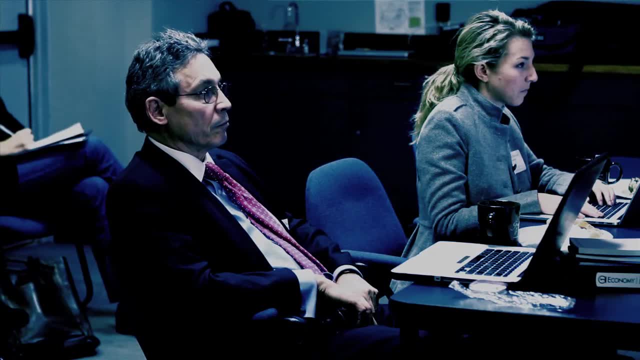 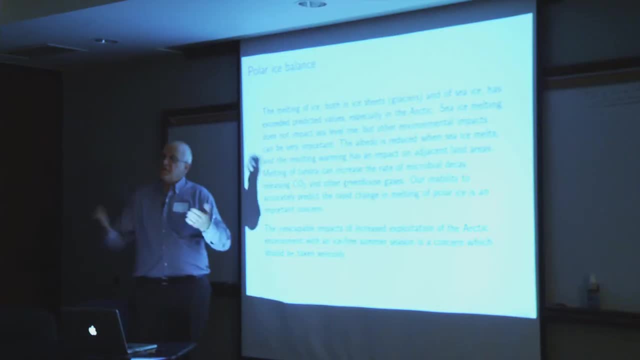 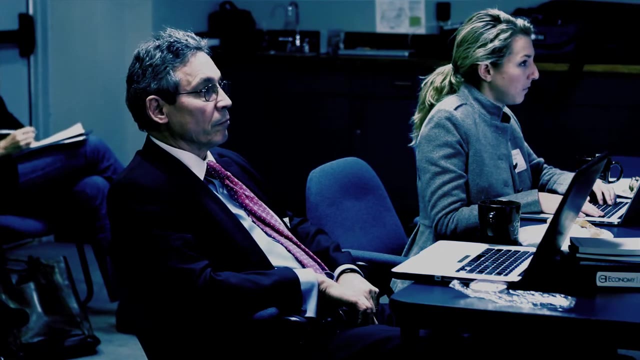 better than if you don't. When you include anthropogenic greenhouse gases in the model simulation, the simulations agree with observations. better than if you don't. OK, so let's talk about some more recent things, things that have occurred since the IPCC fourth assessment reports. 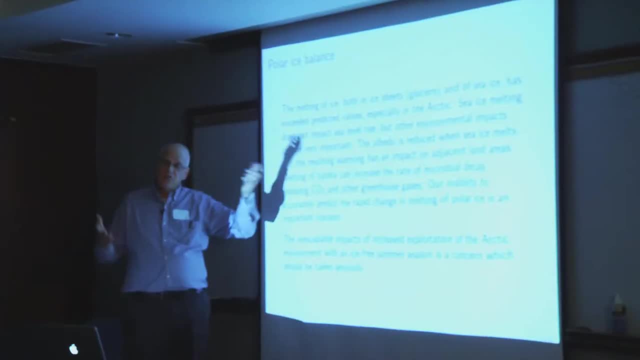 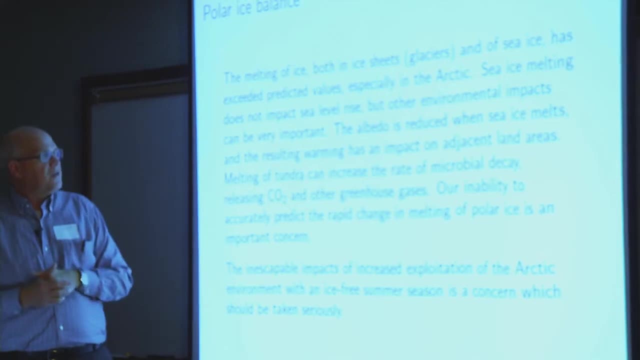 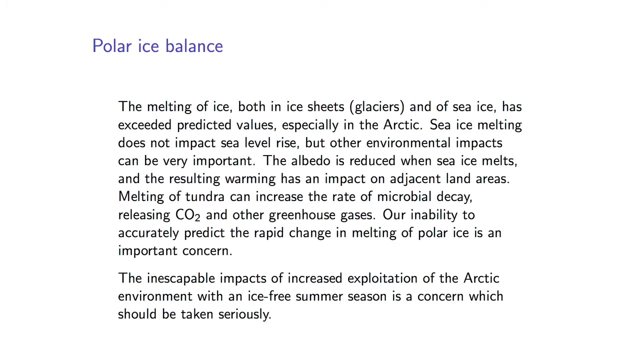 The melting of ice, both in ice sheets, that is, glaciers, and in sea ice, has been much larger than expected, much larger than predicted. The melting rates have exceeded Predicted values, especially in the Arctic. Now, melting sea ice doesn't change sea level. 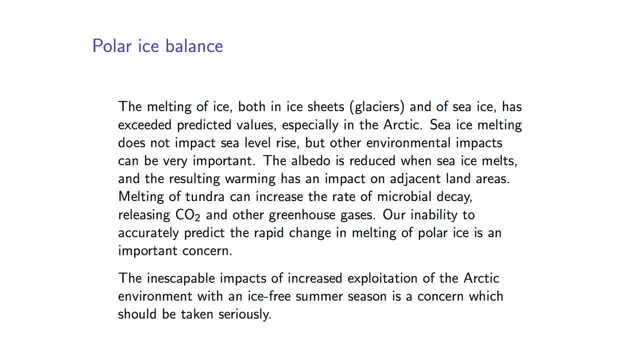 but it has impacts on the environment nevertheless. The ice has a high albedo and reflects sunlight, keeping the environment cool. As soon as the ice melts, the albedo decreases and the heating increases. That can affect both the ocean and adjacent land areas. 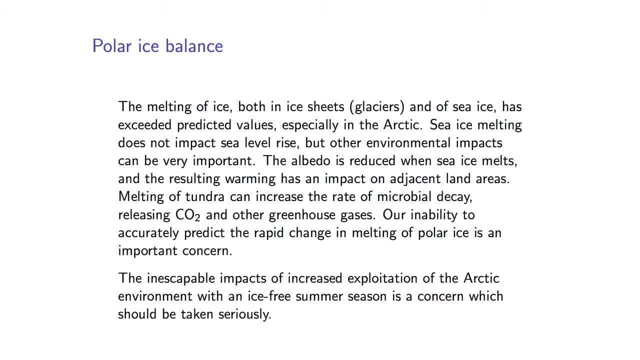 For example, permafrost that's on the land nearby may be warmed by this. Many scientists are concerned about this because permafrost in general contains huge reservoirs of carbon in the form of peat, and also greenhouse gases that are trapped in the ice. 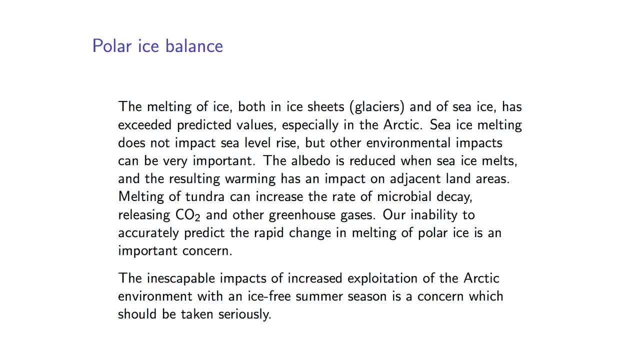 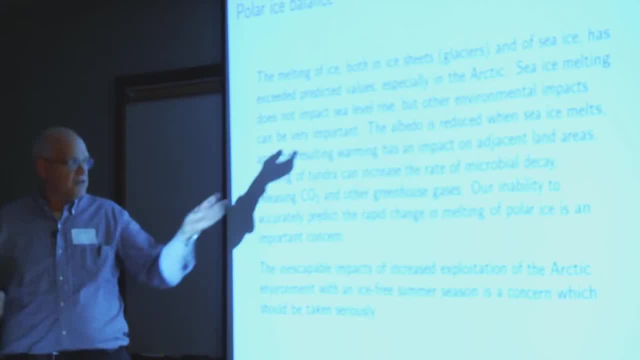 When that permafrost melts, there's increased microbial decay of carbon-rich materials in the peat and release of greenhouse gases. This is a big concern. So even though that's a terrestrial effect, it's impacted by the melting of sea ice. 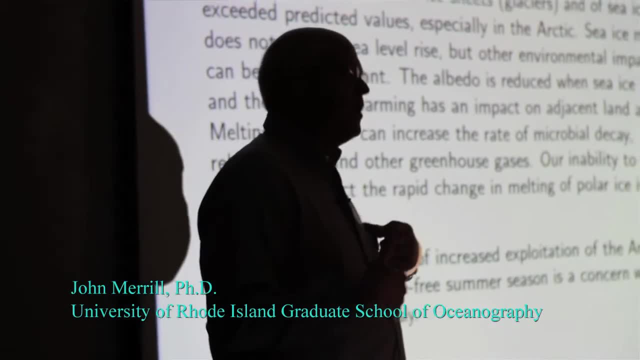 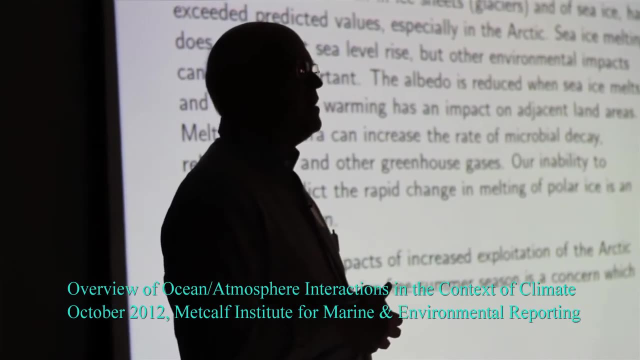 For me, a deeper concern, more fundamental concern, is that we didn't predict this. Our ability to predict melting of ice is really not very good, We're just not very good at it yet. So we didn't predict this rapid change. 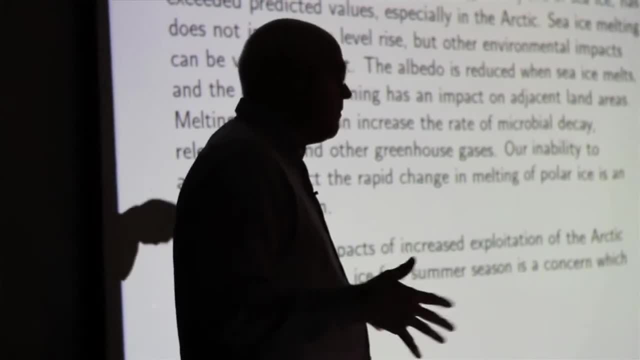 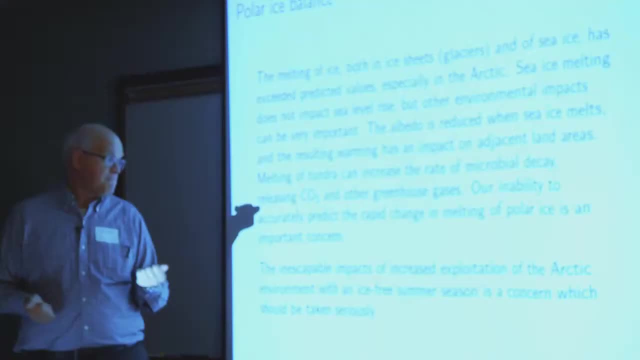 And even though a lot of effort is going into ice modeling, I think our abilities are not as good as they should be, So I'm concerned about that. Now. a lot of space in the press has been taken up on this, And I think it's an important concern. 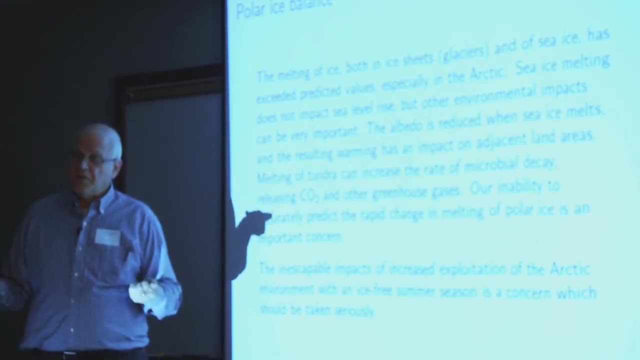 The opening of the Arctic because of the melting of ice there. the potential for having an ice-free Arctic much sooner than expected means we will exploit resources that are there: fisheries, oil and gas under the sea floor. There's going to be environmental impacts. 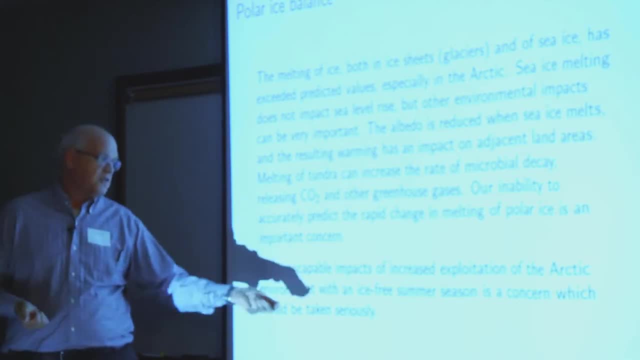 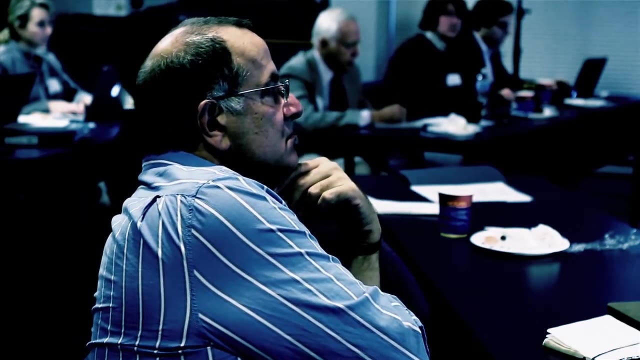 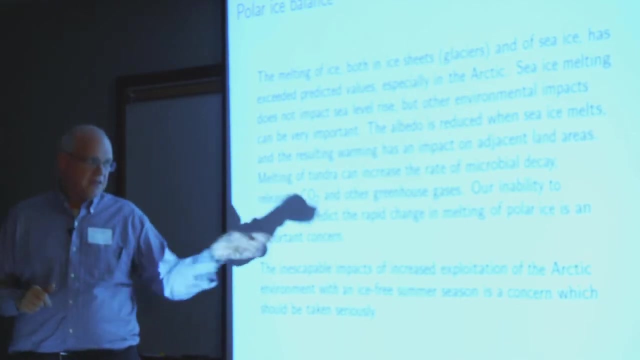 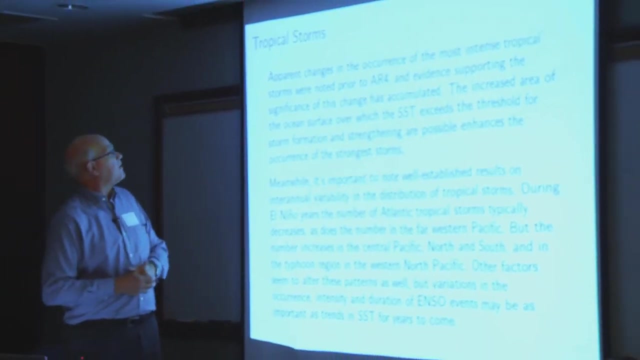 from that kind of exploitation. I think that's a serious concern. The fact that some people are making extreme statements about this should not lessen our concern. We can set aside extreme statements and say: let's be serious about this and take it as an important impact. 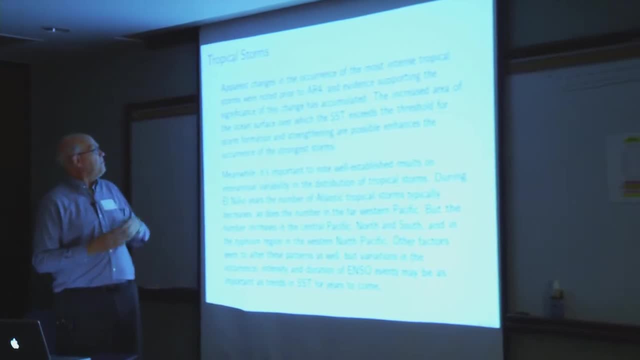 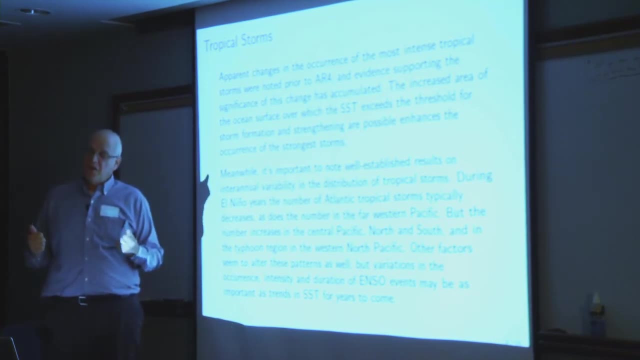 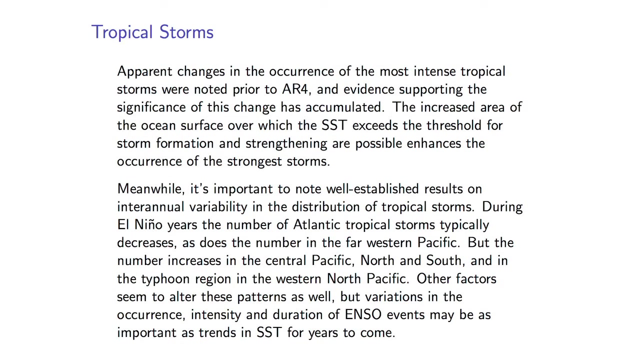 Let's talk about changes in tropical storms. There have been apparent changes in the occurrence of the most intense tropical storms. I'm not talking about increased frequency of storm formation, But a higher fraction of the storms that do occur are very intense, And even though this had been discussed in AR4. 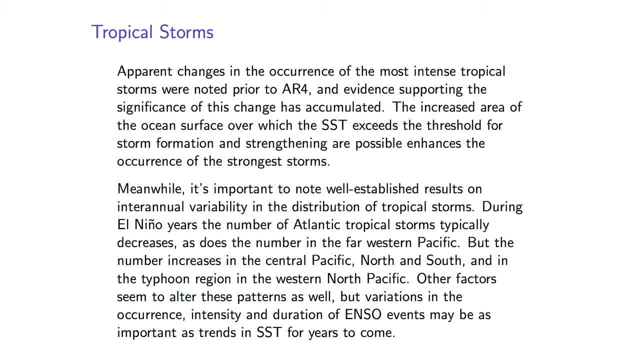 and the idea had been brought out earlier. there's been increasing evidence of this since the fourth assessment report. The idea is that since there's a larger and larger area of the sea surface that exceeds the threshold for tropical storm formation and growth, that means that there's 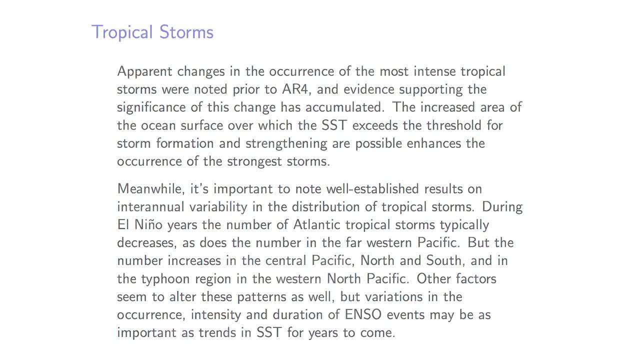 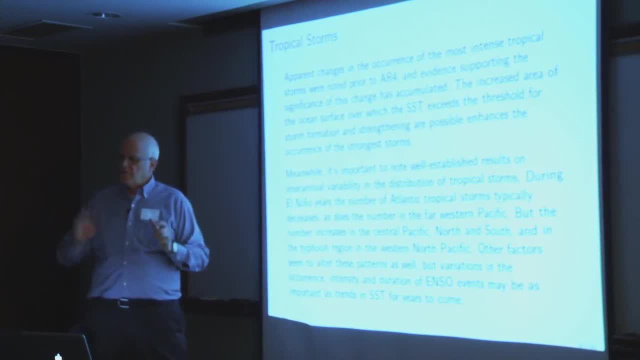 the potential for more intense storms forming. The impacts on coastal environments are widespread and well known, And that's a factor And work is going on both on this campus and in other areas to assess and think about ways in which those effects can be reduced. 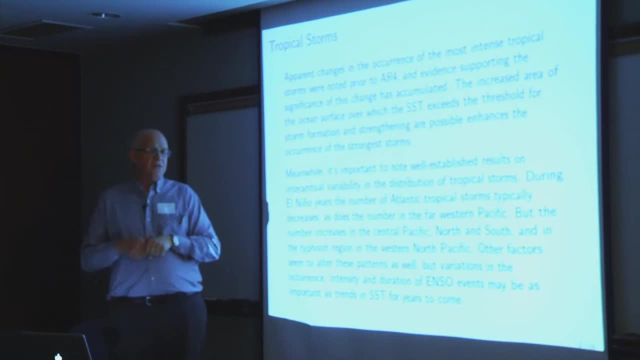 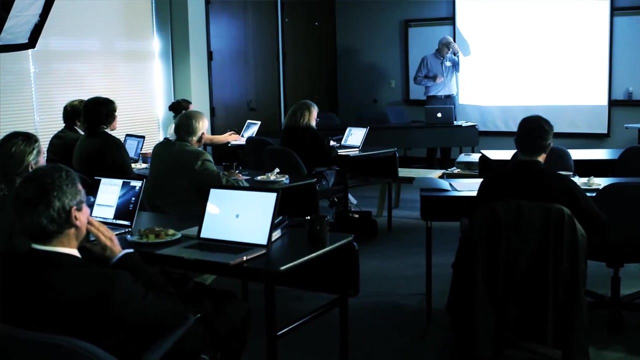 But the most important thing is that these changes are controlled. Now let's talk about- I want to talk about a scientific aspect that's related to tropical storms, but not to the increased occurrence of high intensity storms. There's a natural variability in the occurrence. 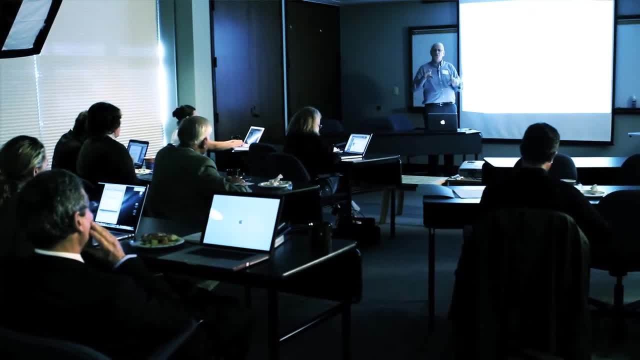 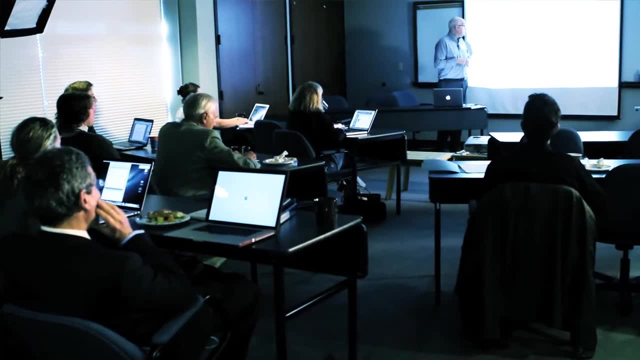 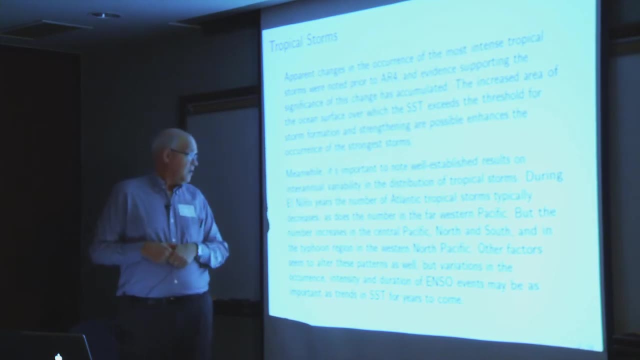 in the distribution of tropical storms During El Nino years. the number of Atlantic tropical storms has reduced. I could give you an hour lecture about that if you'd like, Just try me. But meanwhile in the far Western Pacific there's also a reduced frequency of tropical storms. in an El Nino year, But at that same time in the Central Pacific, both in the North Pacific and the South Pacific, and in the typhoon region in the Western Pacific, tropical storm frequency occurs, increases during El Nino years. 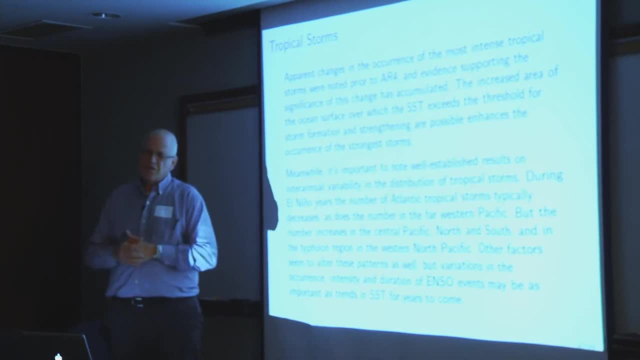 So there's a natural variability in the distribution and occurrence of tropical storms. So what? Why are we talking about this in a thing that has to do with climate change? We've observed changes in the duration and frequency of occurrence of El Nino, events that 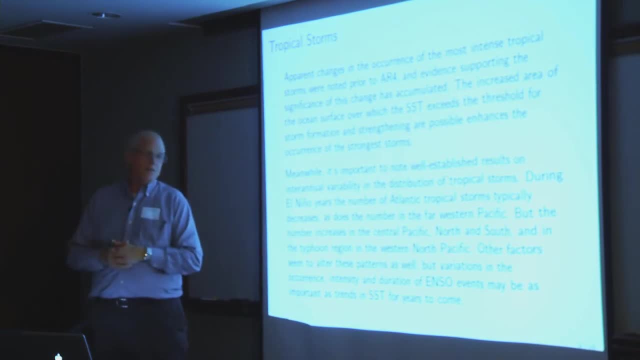 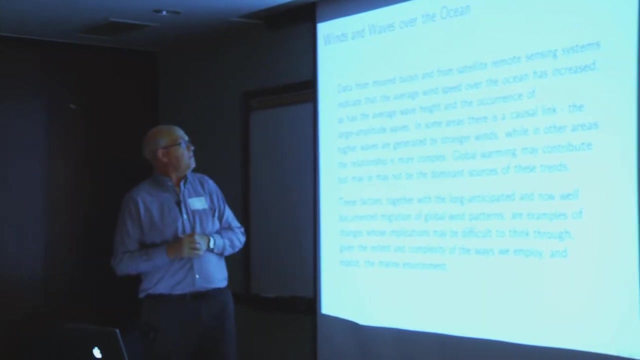 may be related- perhaps not caused by, but may be related to climate change, And that means that the distribution of tropical storms that we're used to could change. We need to be aware of that possibility. OK, winds and waves over the ocean. 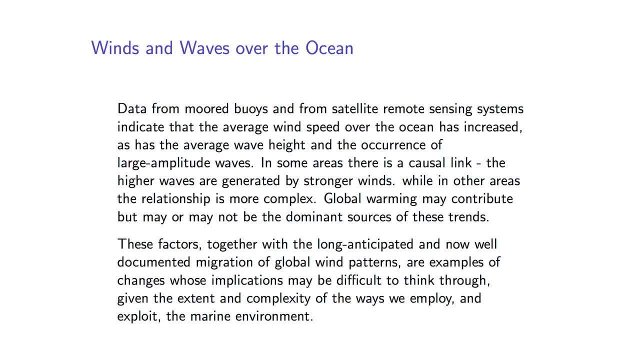 Data both from moored buoys and from satellite observations have indicated significant increases in the average wind speed over the ocean and in the occurrence of large amplitude waves. Surface waves are forced by winds, And stronger winds can mean higher waves. stronger waves. 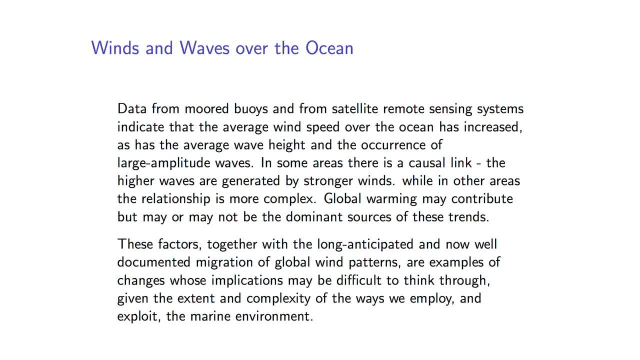 So in some areas there's a causal link. There's a relationship between the stronger winds and the occurrence of higher waves In other parts of the world. there's a link, OK, OK, OK, And maybe there's global warming. 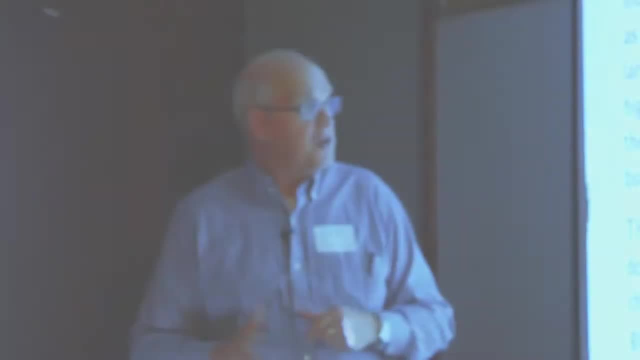 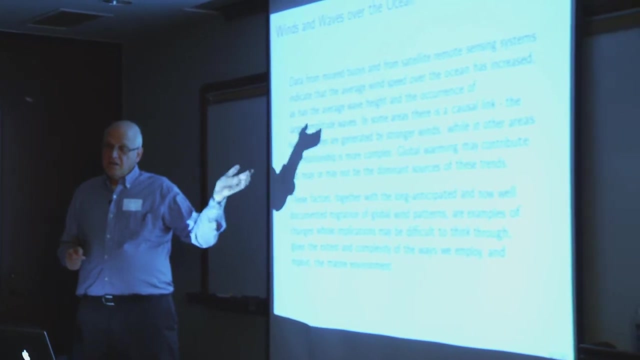 Of course, if there's global warming- and a lot of global warming has awaken in the world- there's not a direct correlation and we're not yet clear what the relationship is Now. global warming may or may not contribute to these effects. 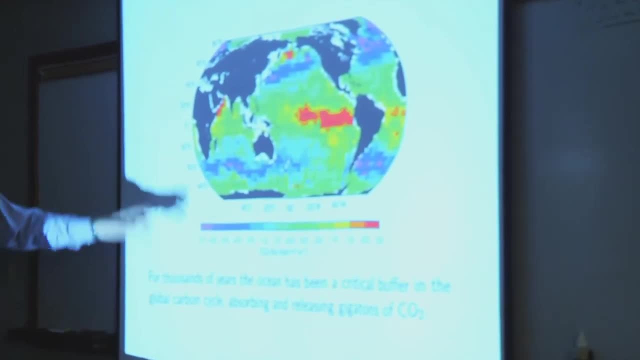 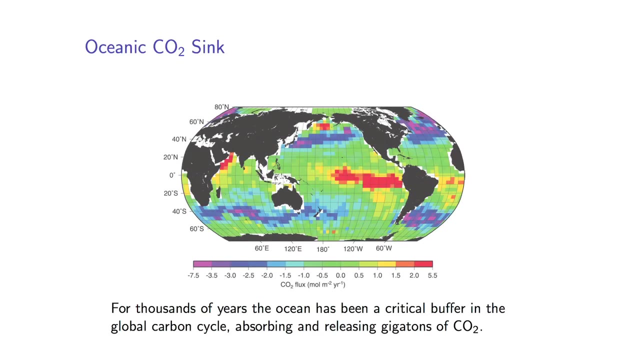 I'm going to run out of time, Okay. so the ocean has been a sink for carbon dioxide for thousands of years. This is a map of the estimated deposition or down-take of carbon dioxide from the atmosphere into the ocean. The tropical oceans emit. 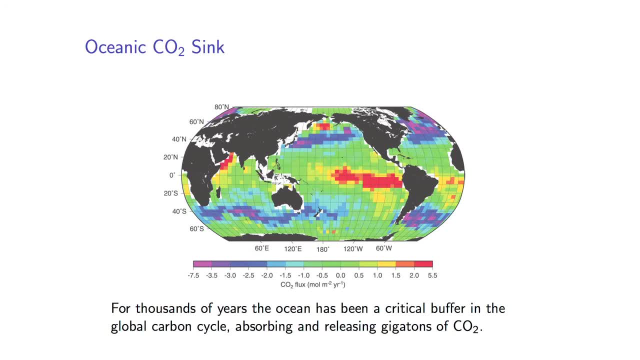 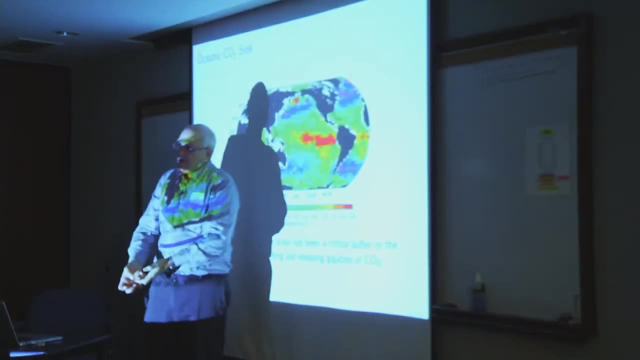 Carbon dioxide. the subpolar and polar seas take up carbon dioxide. That's been going on for millions of years. In the Atlantic, the formation of deep water means that this carbon dioxide-rich water from polar regions is drawn down into the ocean. 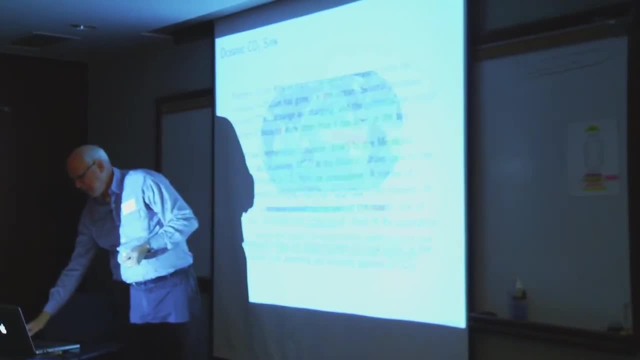 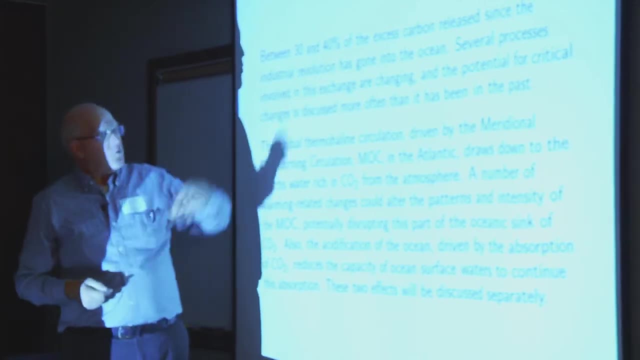 and that CO2 is entrapped. As the environment changes, the distribution of that flux of carbon dioxide changes. So we estimate that between 30 and 30 million years, 30 and 40 percent of the carbon dioxide that we've emitted into the atmosphere. 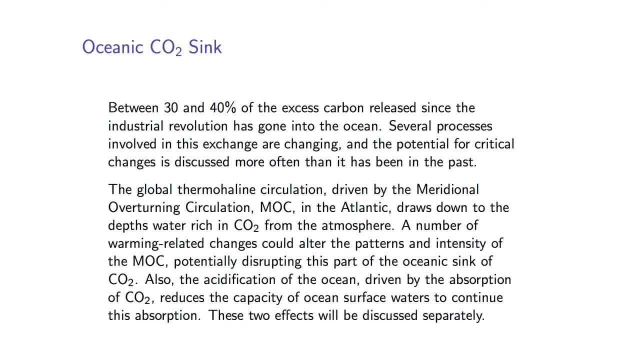 the excess carbon dioxide we've emitted since the Industrial Revolution began. we estimate that fraction has gone into the ocean, But there's a lot of processes that are changing and there's a potential for critical changes. That is it's no longer unusual for scientists to say 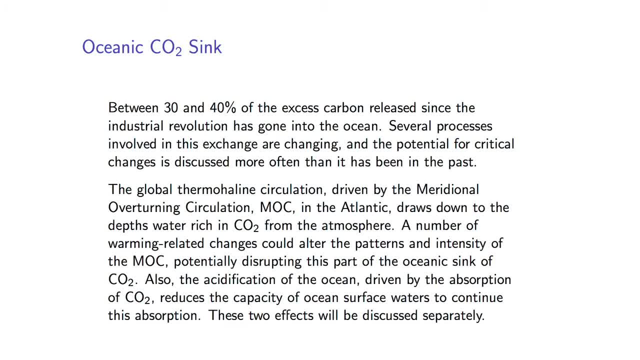 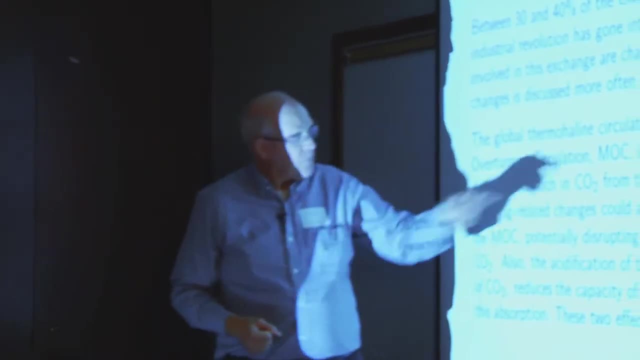 as these processes change, we may find ourselves in circumstances where the drawdown ceases or reverses, The meridional overturning circulation, the sinking of cold, salty water in polar regions that pulls that water down to the bottom of the ocean. 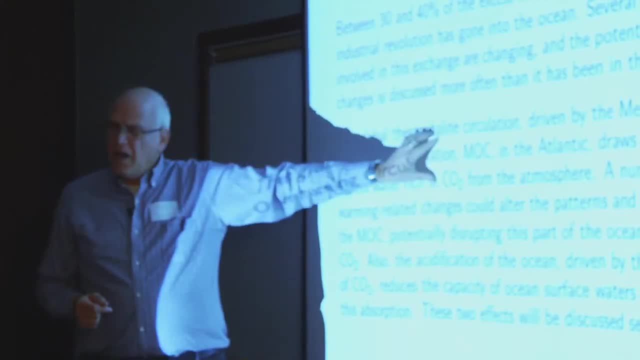 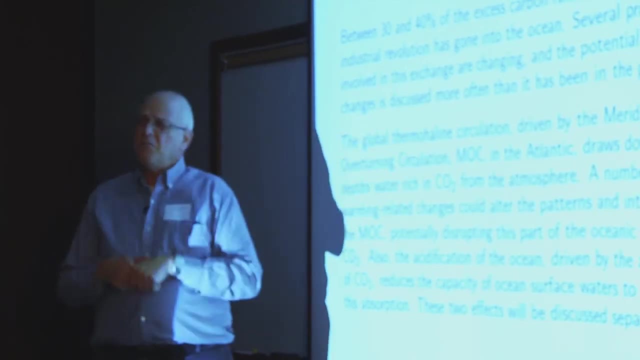 that takes CO2 down with it. The meridional overturning circulation varies in its intensity over geologic time. We don't see any direct evidence that the meridional overturning circulation has slowed, but that potential does exist and that's something that we need to look into. 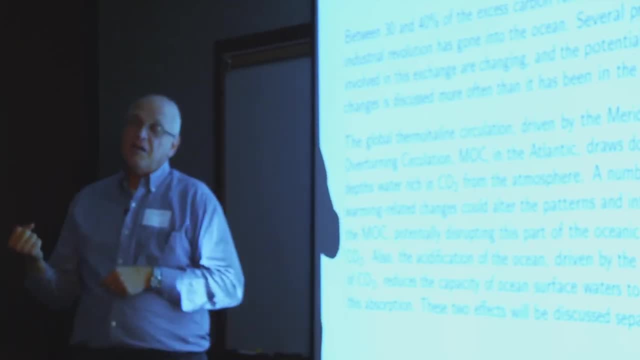 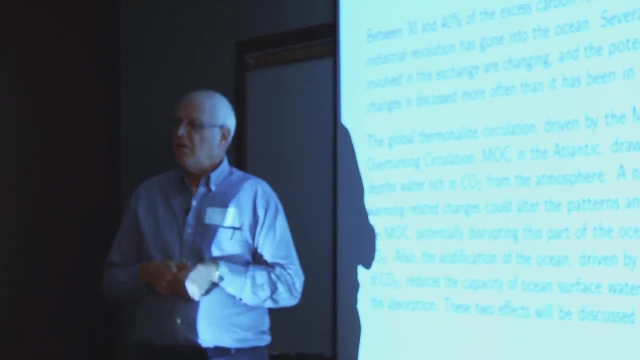 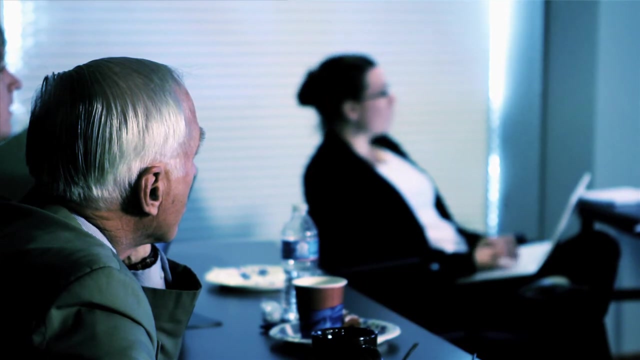 The acidification of the ocean means that its ability to take up carbon dioxide from the atmosphere by the physical chemical processes that changes as the ocean is acidified and so the capacity of ocean surface waters to take up carbon dioxide is changing. I want to talk briefly about things related to the ocean. 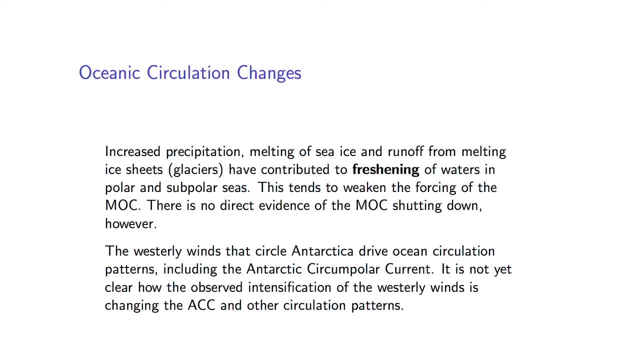 That tends to weaken the formation of the meridional overturning circulation, because the water at the surface doesn't as easily find itself in highly saline, very cold conditions. Again, I'm not arguing that the MOC is shutting down, but there will be changes in the circulations. 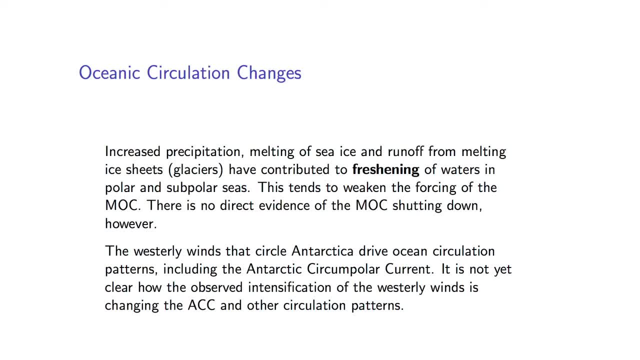 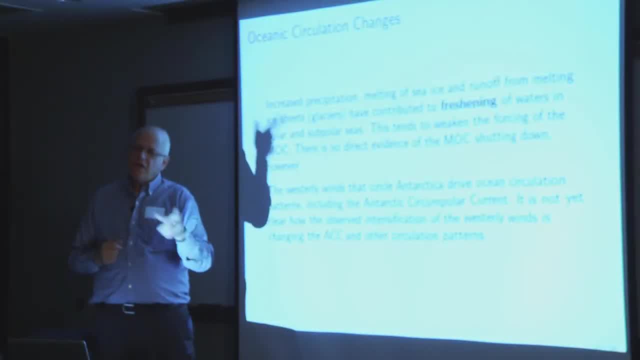 caused by these rapid changes in the environment. In the Antarctic there's a westerly wind. There's a wind from west to east that drives an Antarctic circumpolar current. That current is an important mediator of ocean chemistry and there have been changes in this circulation. 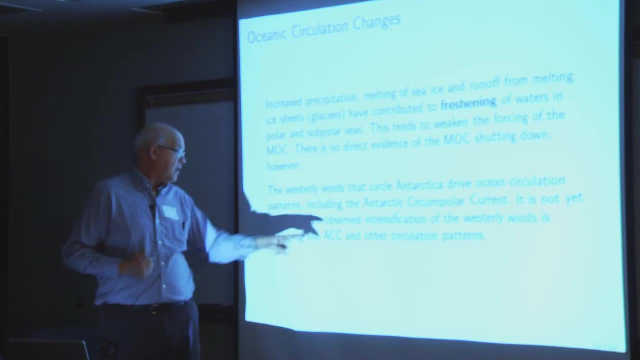 and observations are being made and analyses are being made, But that's an example of a place where there's an important role that the ocean plays and, as the circulation both of the atmosphere and ocean changes, we need to accelerate our studies to understand the implications of the changes that are occurring. 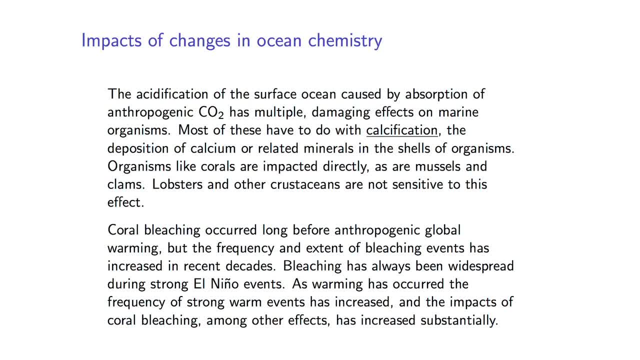 Very quickly. you're aware that ocean chemistry is changing. The ocean is becoming more acidic because of the uptake of carbon dioxide. There are a lot of organisms that rely on ocean chemistry to build the shells that they live in, and so the business of decreased calcification. 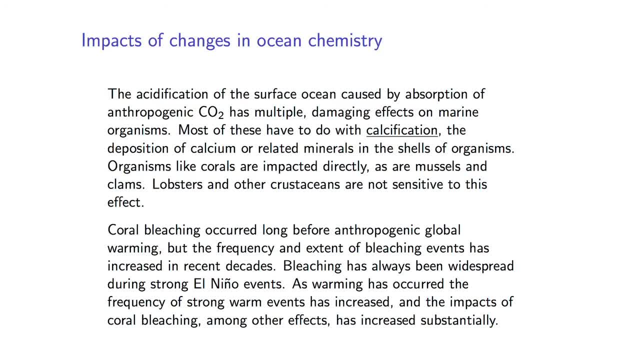 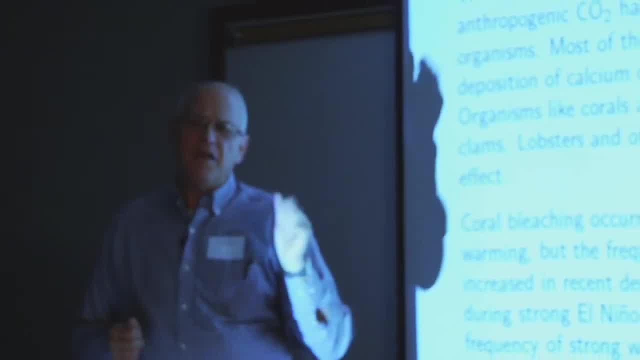 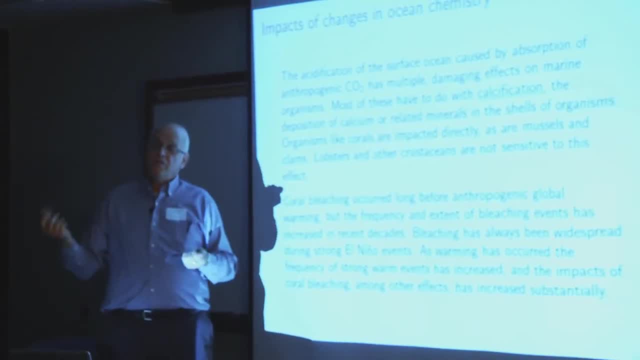 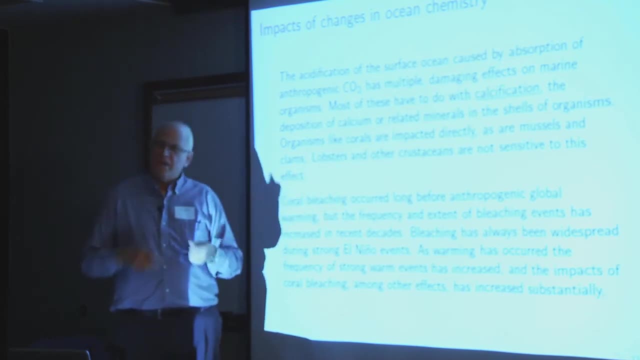 is a serious concern. I summarize here that crustaceans are not directly affected by this, but mollusks are, and of course, you're aware that corals- calcification in corals- has been raised as a significant issue. Coral bleaching occurred naturally. 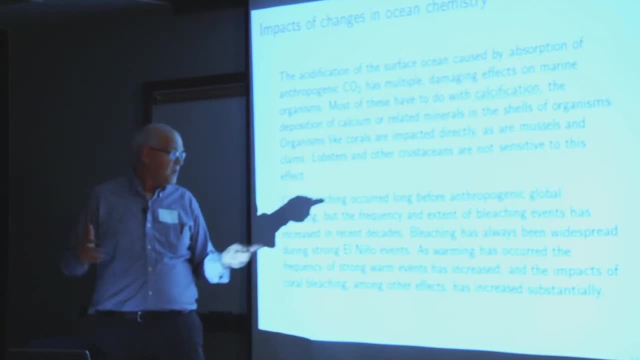 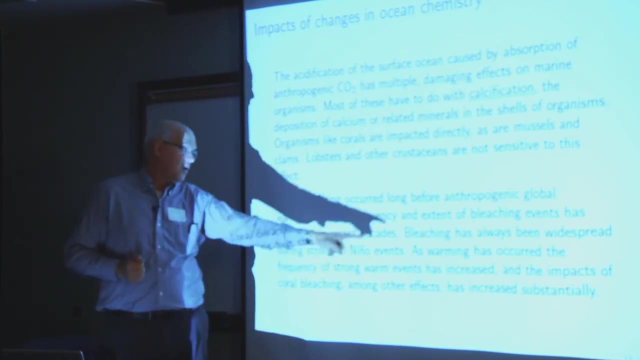 long before anthropogenic global warming took place, but bleaching has increased in its frequency and intensity, and that's a concern. Bleaching has always been widespread during El Nino events, but again, with increased acidification of the ocean, the bleaching has become a bigger concern. 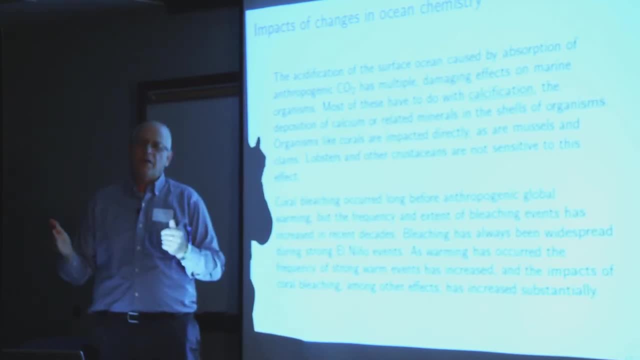 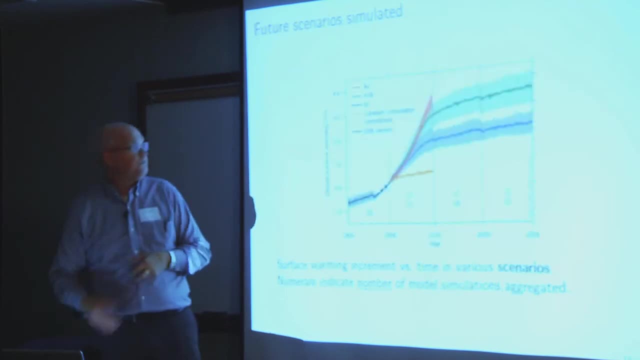 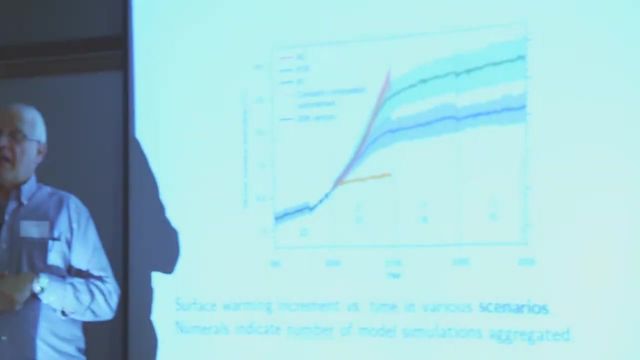 and as the occurrence of El Nino, events has shifted with global warming, there's evidence that the extent and duration of bleaching has increased as well. We're getting towards the end of what I want to say, and these are climate simulations going into the future. 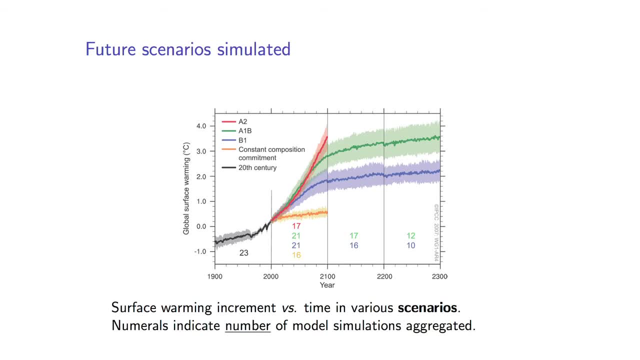 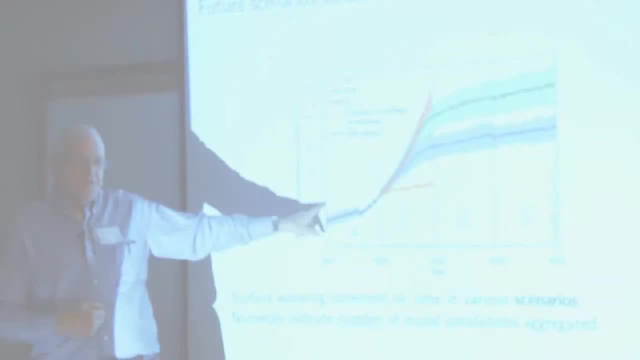 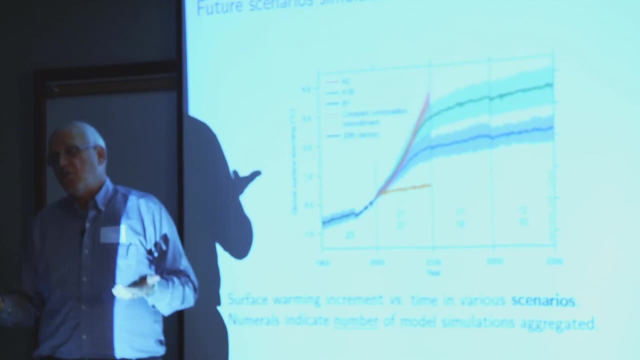 So this is again a figure from the fourth assessment report and it shows the record of global warming up to the global average temperature from 1961 to 1990, and then shows projections into the future, making different assumptions about the way in which humans will deal with the environment. 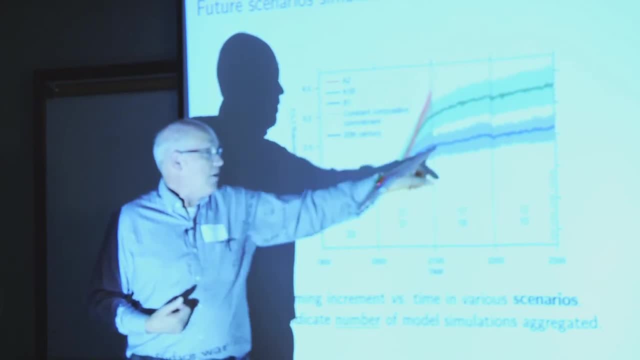 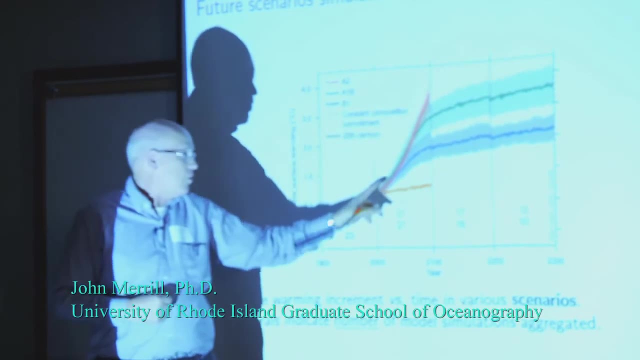 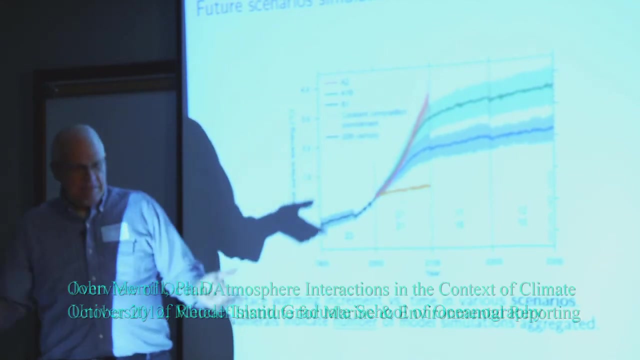 You know, a steady-as-you-go change, or a rapid implementation of emissions controls, or I think someone might say this would be the European model. you know, cut down everything, tax, all that leading to eventual stabilization of the global warming. 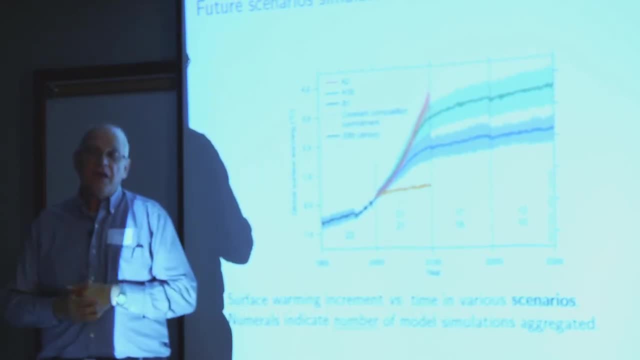 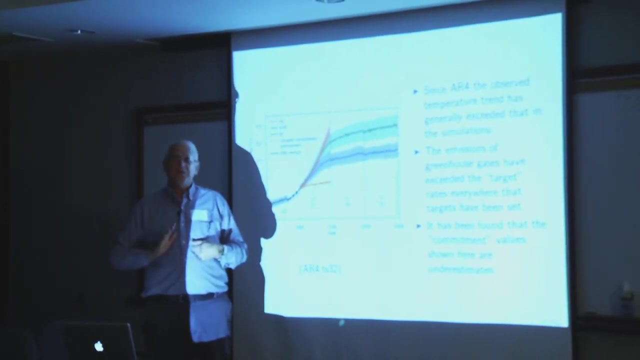 Scientists have been aware for a long time that even if we stopped emitting greenhouse gases yesterday, we've already committed to a significant climate change because of carbon that's already in the environment. I've got three pretty pointed remarks. This is in part my opinion. 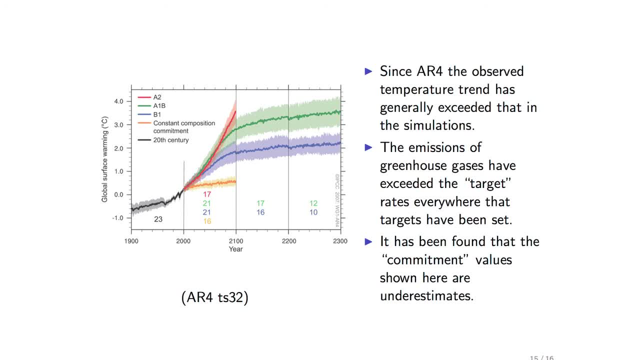 The observed temperature trend has generally exceeded the simulation results, That is, the simulated results are not extreme. Scientists have been conservative in promulgating those results. The emissions of greenhouse gases: where we have tried to control the emissions, we've not succeeded. 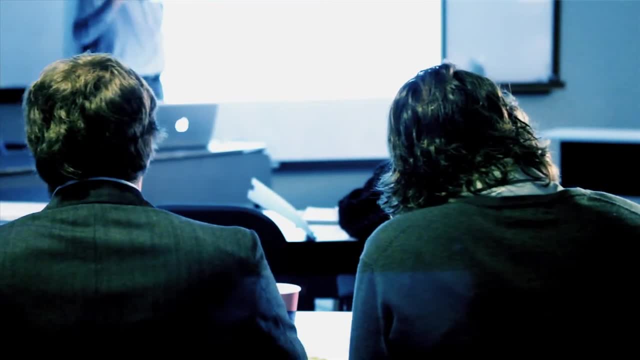 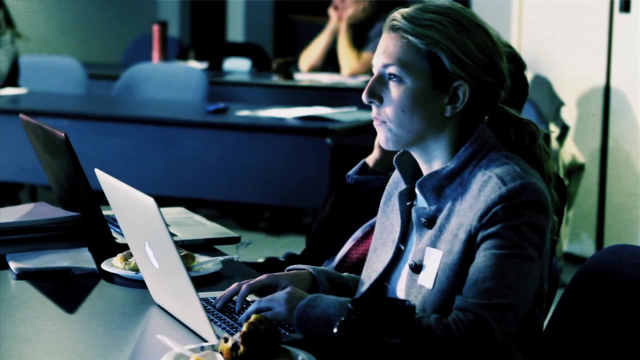 No matter what mechanism we've used to try and control emissions, I'm not aware of any place in the world where emissions have fallen below the targeted amount. We set a target. We say: well, let's do these things to try and reduce our emissions. 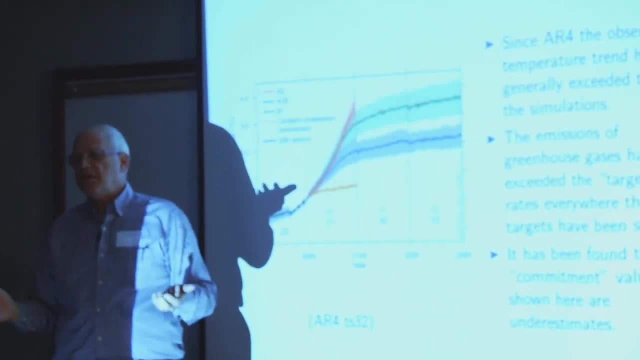 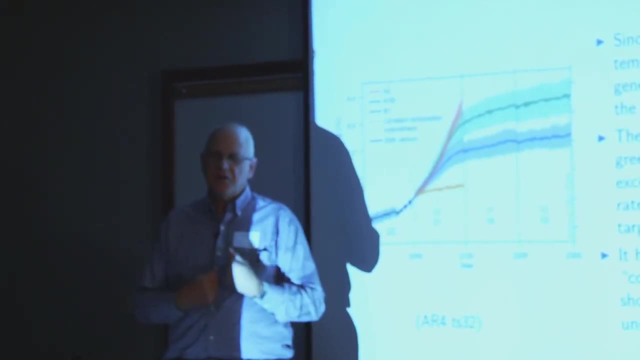 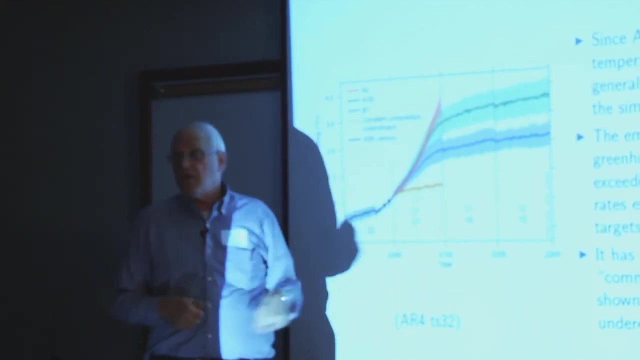 And then we tax, we regulate, we do all kinds of things. Somehow the emissions still exceed our targeted amounts. This is not good news. The commitment, the committed climate change that's shown here, it's wrong. The new estimates show the committed climate change is higher than this.